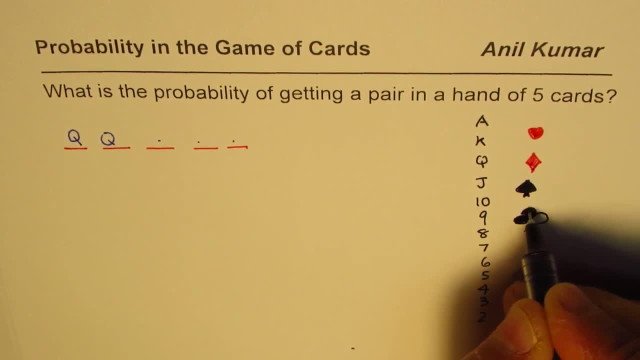 So these are the four suits, So every card. for example, we'll have four aces, four kings, kind of like this. So four times 13 will be 52. So what we have here is 52 cards. Those are total number of cards for us. 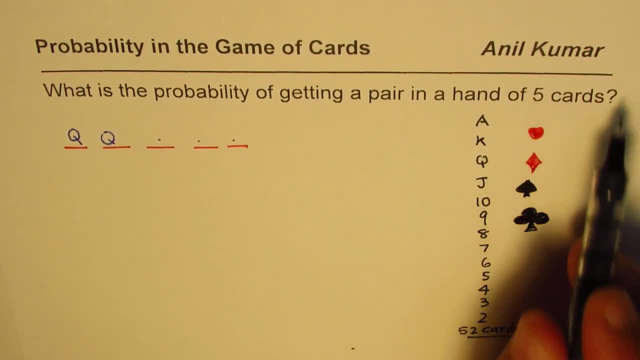 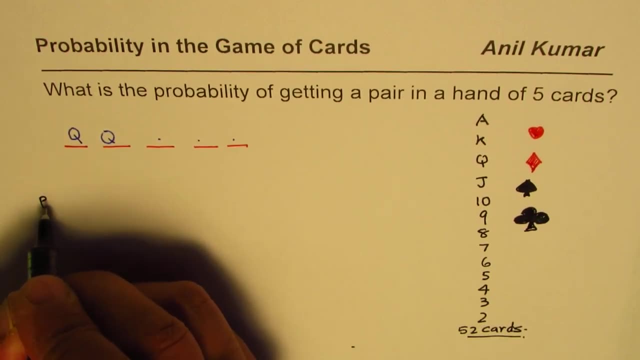 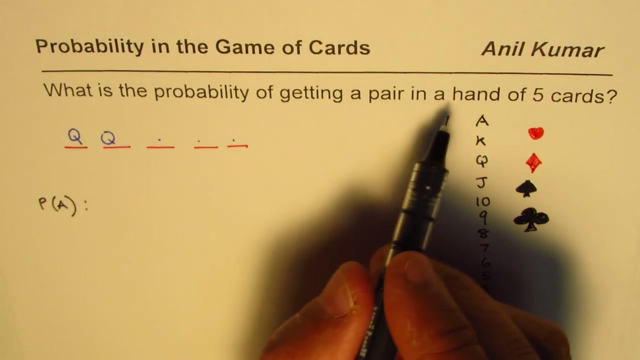 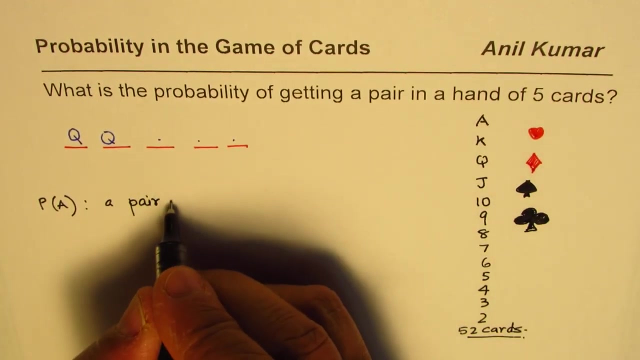 Okay, So when you're drawing five cards, in that case, the probability will be, so let's write probability of doing this event, which is event A. Event A is getting a pair in five cards. So that is what we need to find. 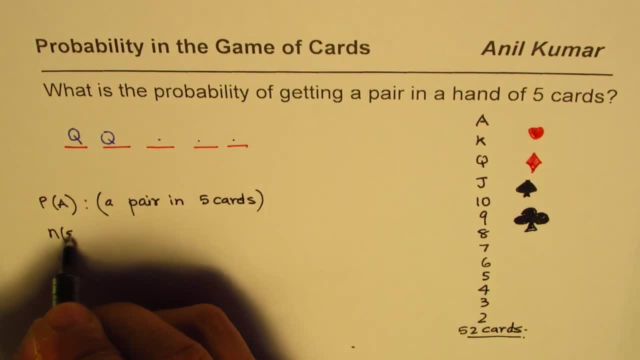 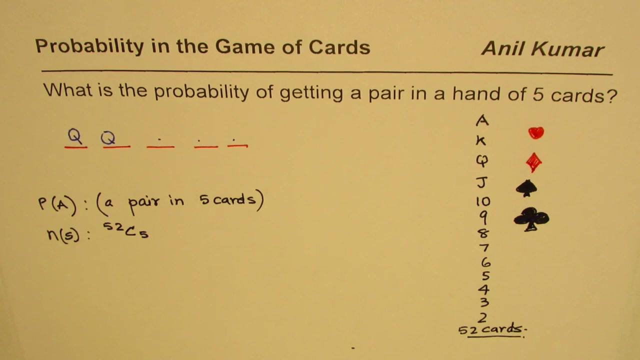 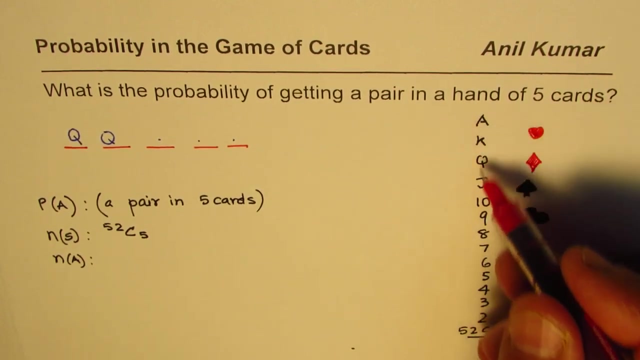 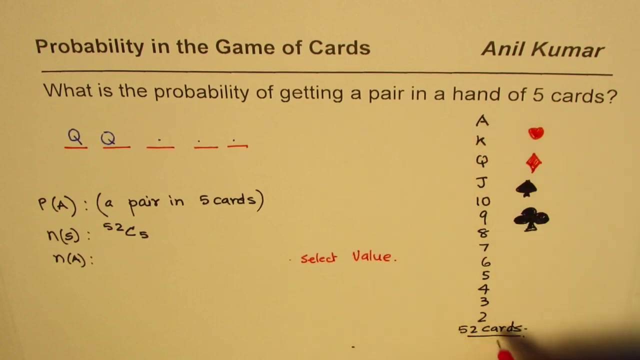 Now, here total number of options are. we have to choose five out of 52 cards, So it is 52 C5, right, Right, Order is not important. Order is not important here when you have a hand of five cards. So that is total number of options. Now we need to find what are favorable options to get a pair. So the first step here is to figure out what value of card you need and how many options do we have to select value. So first thing is, let us select value. Now, since there are 13 cards, we have 13 choices. So we have 13 choices. 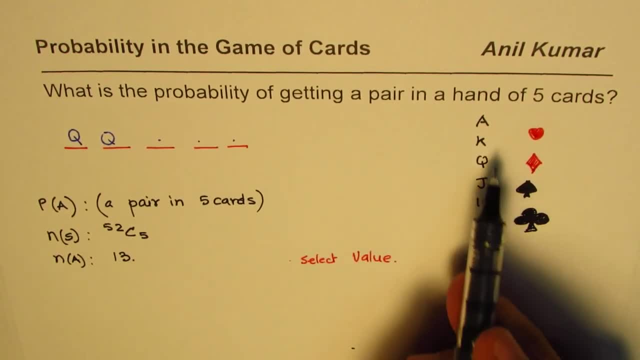 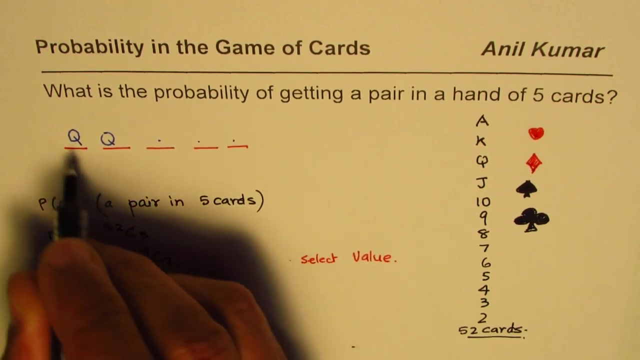 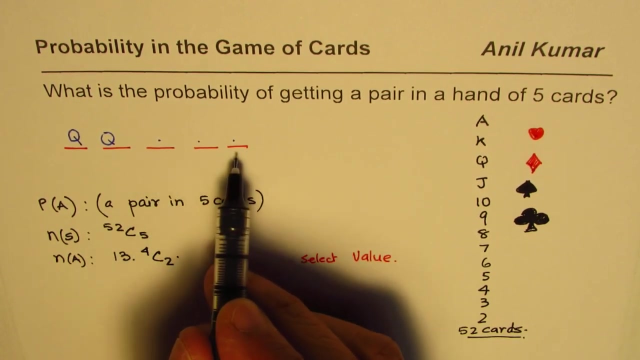 Now, out of these 13 choices we want two of the same kind. As you know, if we select Q, Q in, there are four of these. So we have a choice that out of four we could select two right. Out of four we could select two queens, So that becomes a pair. Now the other three cards can be any card but not Q right, But not the queen. Otherwise this will no longer be a pair. So we have to figure out what are favorable options to get a pair. So that is total number of options. 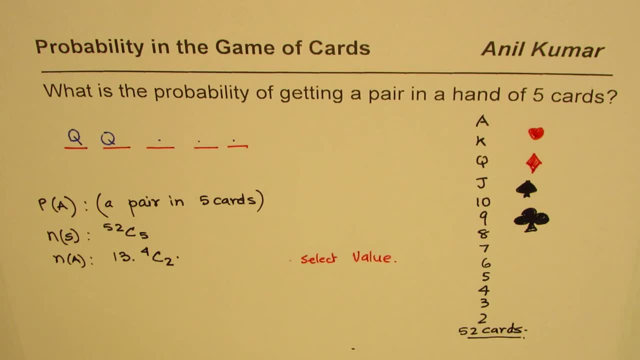 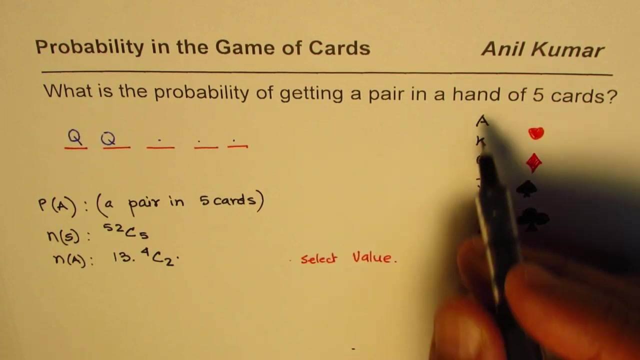 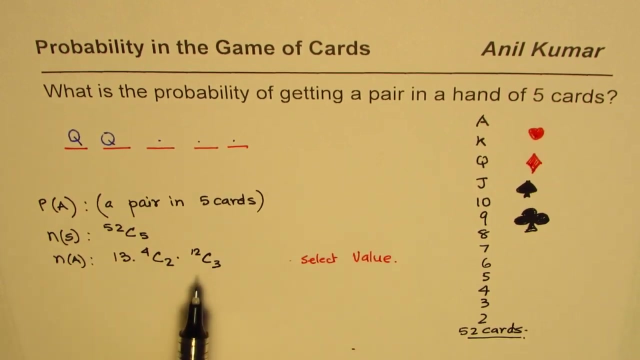 So now we have to select three cards out of remaining 12.. Do you understand? So out of remaining 12, we have to select three cards, So that becomes out of 12, we have to choose three, And these three, whichever we select, will be of any of these three.